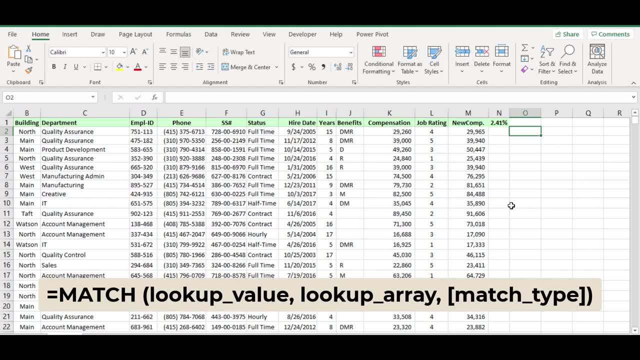 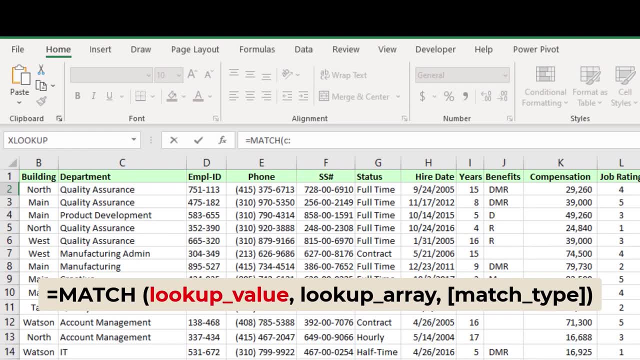 So I will use excel match function to return me the location where it will be returned, the first occurrences of the department names. So match lookup value will be C, colon C. Then for the lookup array argument also I will use the same range. 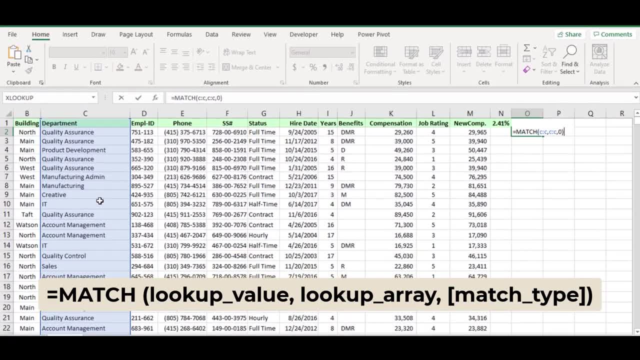 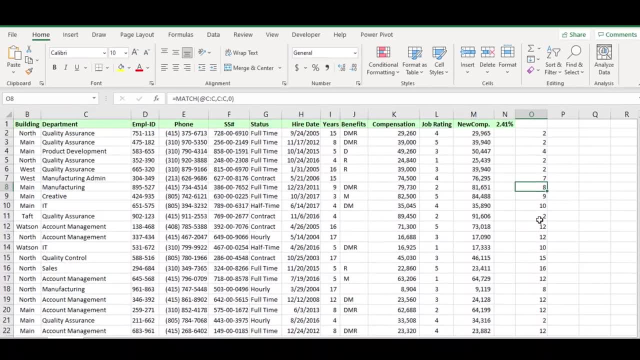 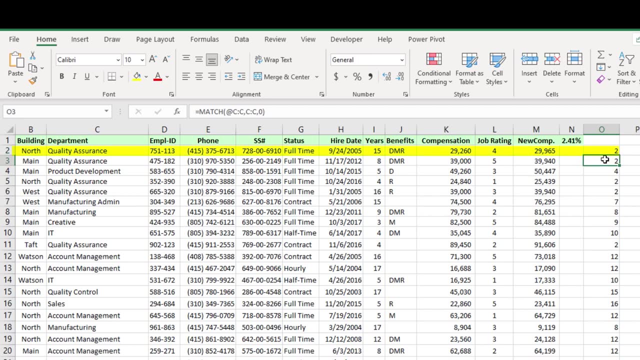 C, colon C, with exact match. Now copy down the formula. Now the formula is returned. the location of the first occurrence for each department name: C: the quality assurance department name: The first occurrence appeared in row number 2. And it has repeated in the next row and continue till complete entire dataset. 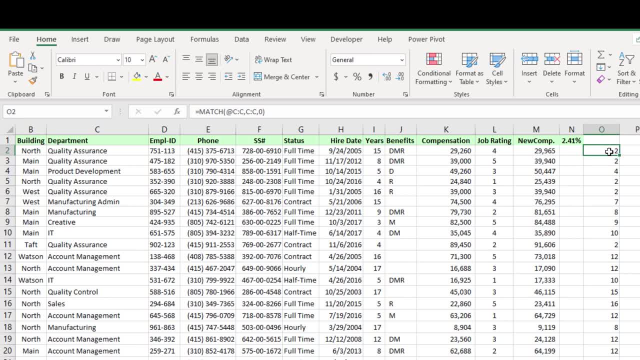 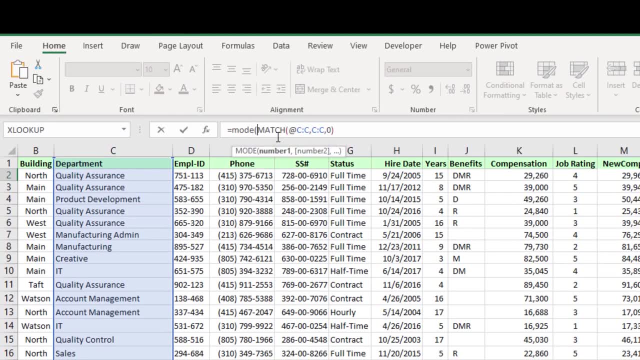 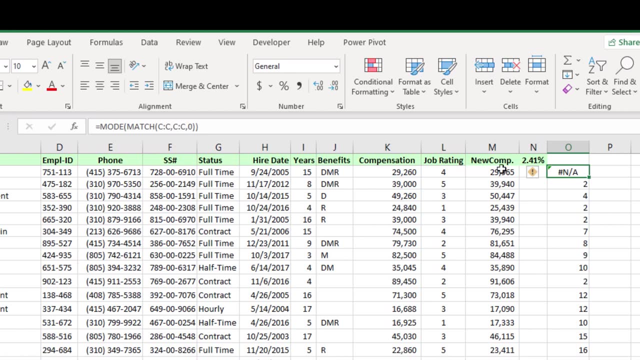 Okay, Now we have converted the department names to a number format, So we can use the excel mode function, Hence mode. leave the match function as the number range, Then close the bracket. Now the formula has returned me the error value. This is because of the counting blank cells. 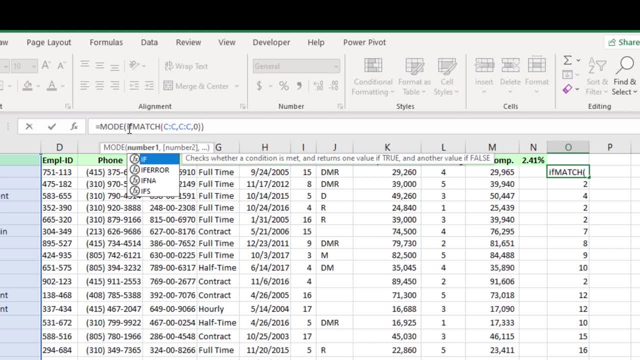 So I will use if function to omit the blank cells. So before we use mode function, let us use if function. Hence, if The logical argument will be C, colon C, not equal to blank, Then leave the match function as true value. Leave the false argument as default And close the bracket. Okay, Now the formula has returned me the number value 8.. It means the department name at the location 8 recruited highest number of employees. To return the name, instead the location number. 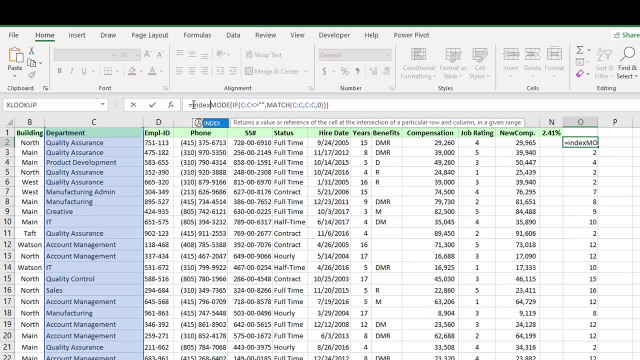 Use the index function, So index array argument will be C, colon C. then leave the mode formula as row num argument, Then close the brackets. Now the formula has returned the department name, So the manufacturing department has recruited highest number of employees. 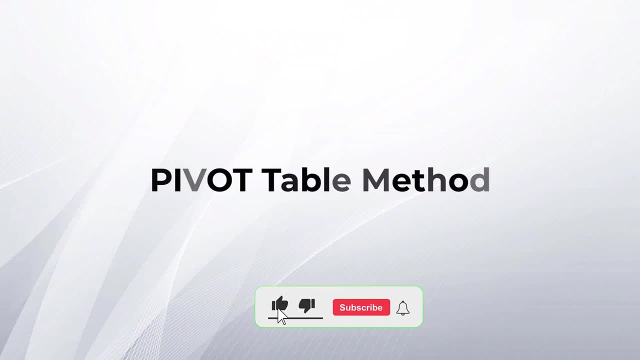 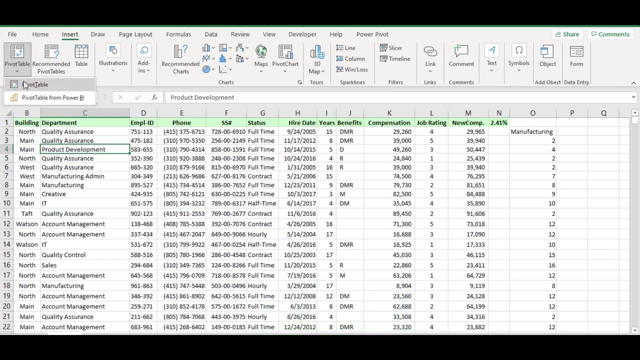 Okay, Next let us use the pivot table method. Click on any cell in the data table. Then go to insert tab And choose pivot table option from the drop down. Next choose the option to create the pivot table on the existing sheet. 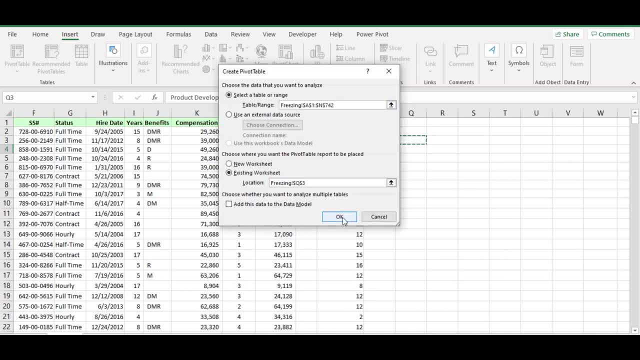 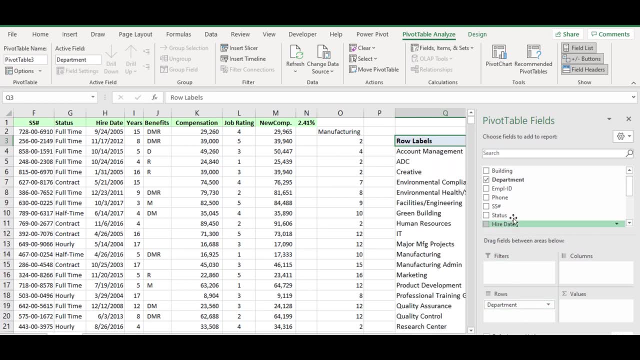 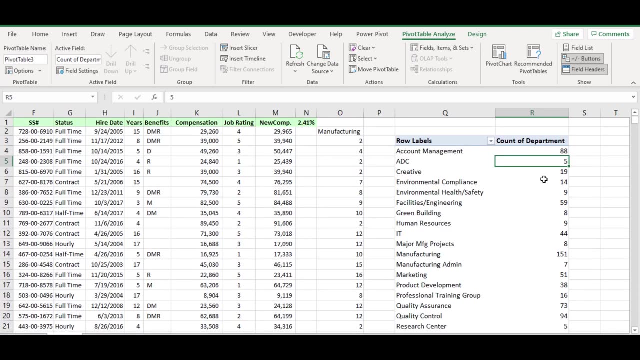 And select any cell as the pivot table location. From the pivot table pane, Drag and drop the department field to the rows area. Again, drag and drop the department field on the value area. Now the pivot table is created. Next, right click on the count of department column. 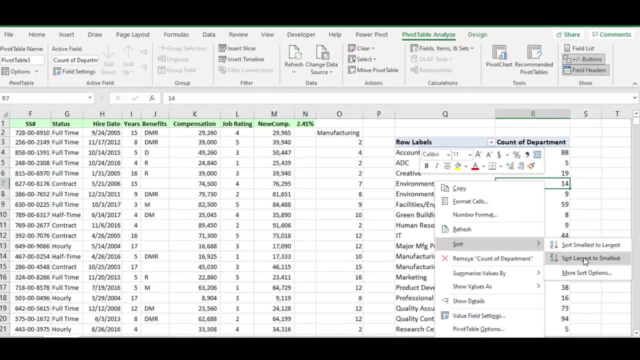 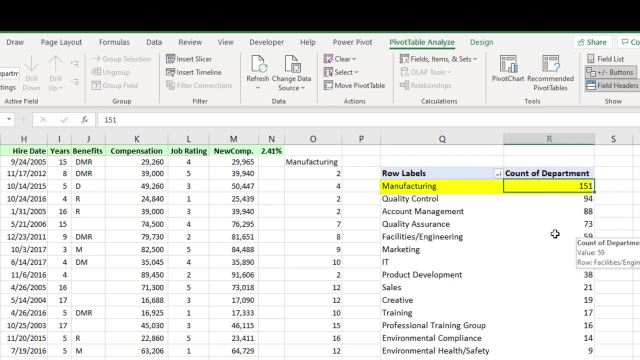 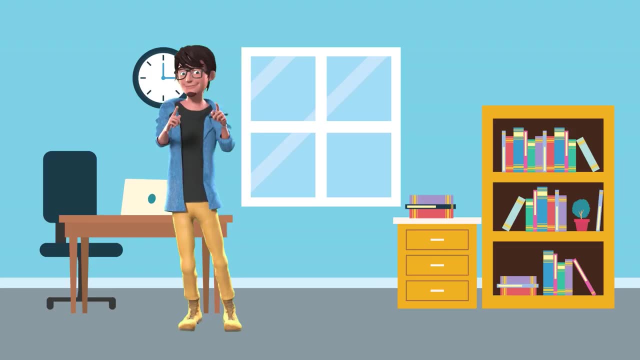 Expand the sort option And click largest to smallest From the table. the manufacturing department name is brought on the top, Which has recruited 151 number of employees. So in both methods we got the same department name. So I hope this lesson was useful for you. 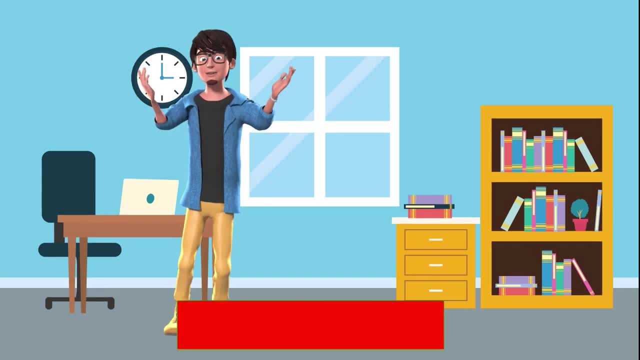 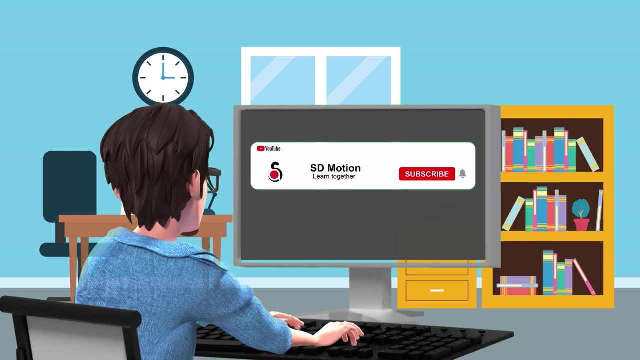 I will see you in the next video. Thank you for watching. If you have any comments on this lesson, Please mention in the comments section And make sure to like the video And consider subscribing to my youtube channel for more future videos. Have a nice day. 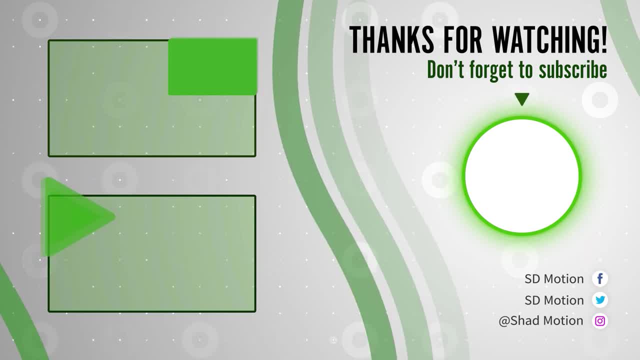 See you in the next video. 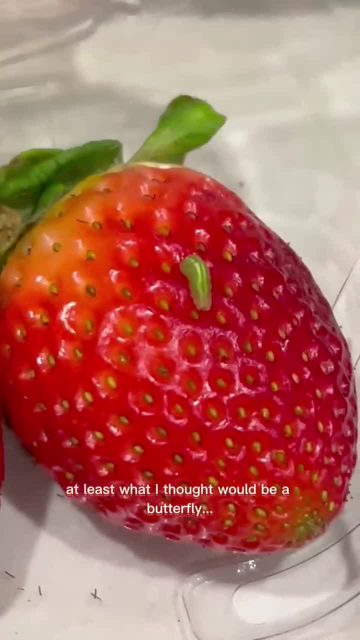 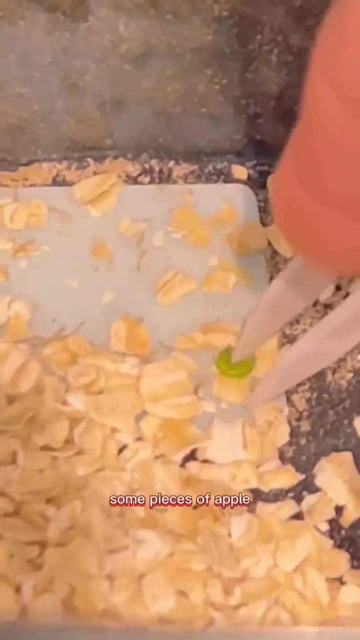 I found a bug on my strawberry and grew it into a butterfly, At least what I thought would be a butterfly. I took the little green caterpillar and put her in my little animal kingdom, Added some oats, some pieces of apple. I was determined to be a very good caterpillar. 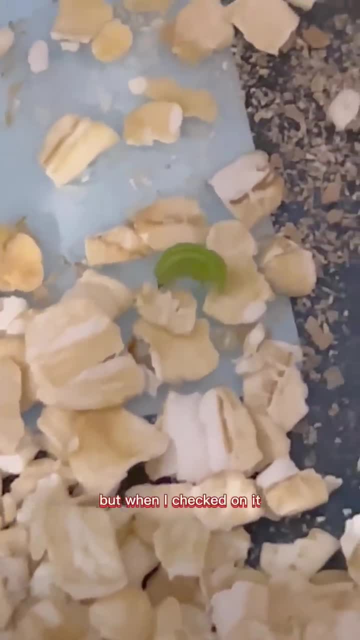 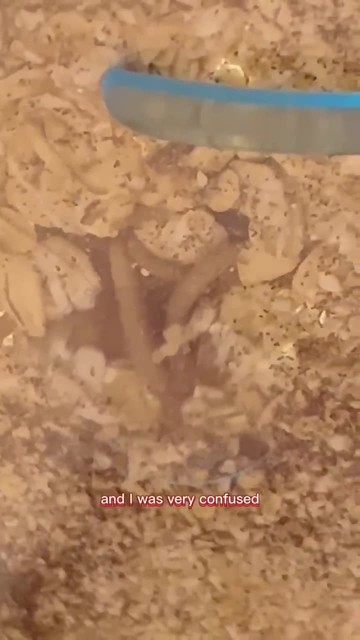 mother and I waited a few weeks for something to happen, But when I checked on it, I saw that there were numerous little bugs- and they weren't green caterpillars- and I was very confused. I started to watch these little bugs morph into something other than a beautiful 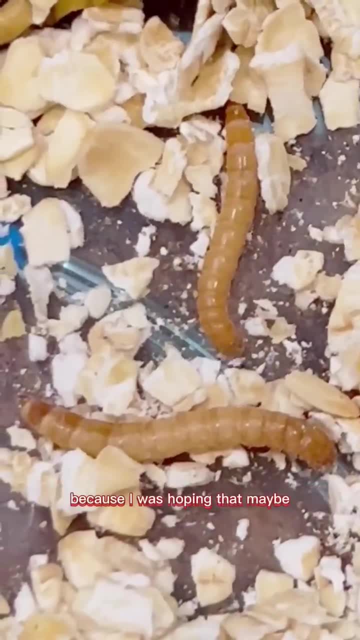 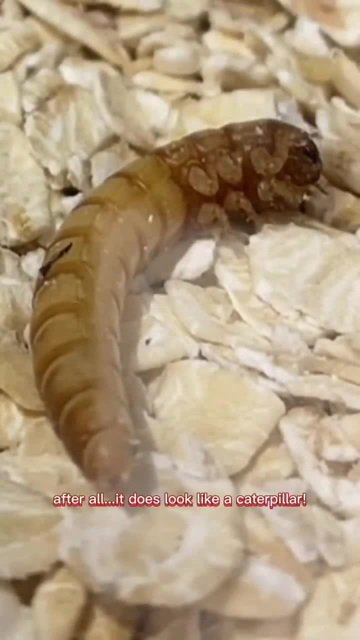 butterfly. I was itchy looking at these things and quite confused, because I was hoping that maybe that little green caterpillar had babies and we would have a hundred butterflies instead of just one. After all, it does look like a caterpillar, right? Right, So to prepare. 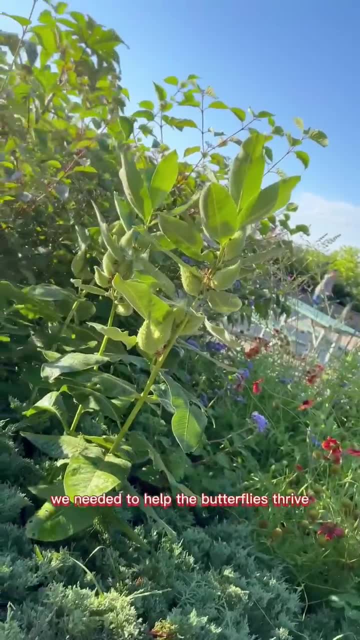 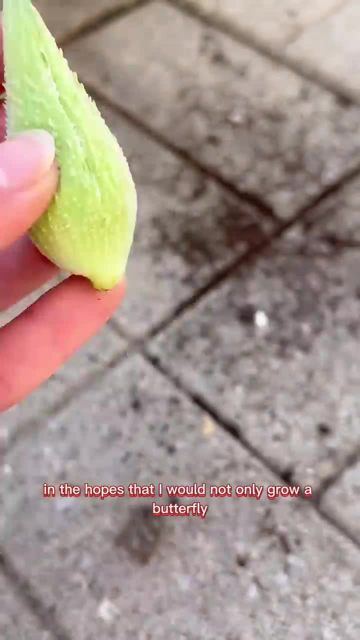 for the birth of our butterflies. I did a few things We needed to help the butterflies thrive. I got some milkweed seed pods- the host plant for monarch butterflies- to lay their eggs on, in the hopes that I would not only grow a butterfly but also have that butterfly. 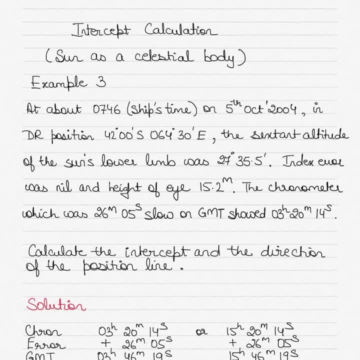 Hi guys, today we'll take up a new question in the area of intercept calculation and also calculation of the position line or orientation of the position line. Today we'll be using sun as an example of a celestial body. You can find the links to the previous examples in the